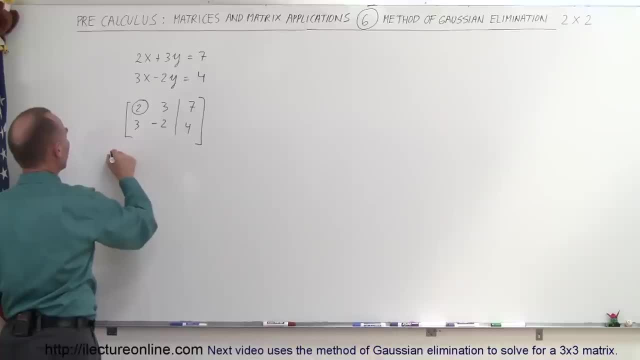 do that by dividing the first row by two. so row one is going to become one half. I'm simply going to divide that row by two. When I do that, I get the following matrix: I end up with a one, a three halves, a seven halves, and the second row is unchanged like. so The next thing. 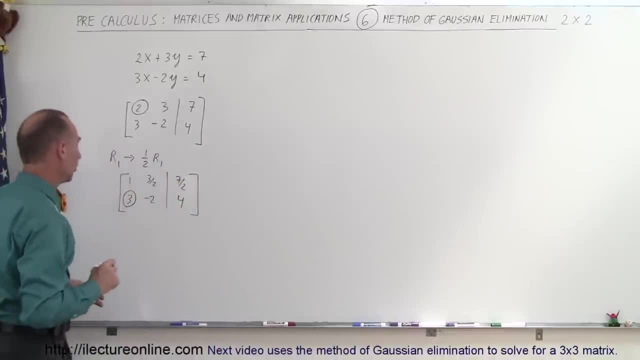 I want to do is turn this into a zero. I can do that by simply multiplying the top row by the negative this number and then adding it. In other words, row two will become negative three. at the end, I take the negative this number, multiply it times the row with the one in it and adding. 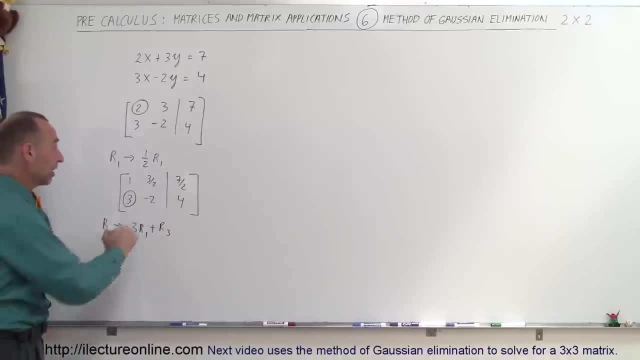 it two, row three, to eliminate that three, to see what happens. Of course I need to do the same to everything else in that row. So that means the matrix will now become as follows: The first row does not change, So I get a one, a three halves, a seven halves, But here negative three times one. 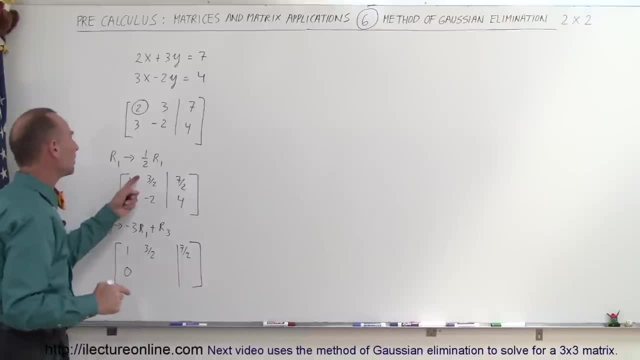 added to three, gives me zero Negative three times. this gives me a minus nine over two. Added to negative two, that's another minus four, OK, to minus 13 over 2.. So again, negative 3 times. this gives you minus 9 over 2, and add it. 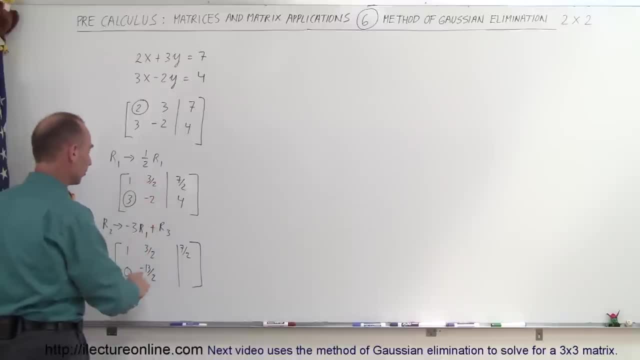 to minus 2, that's a minus 4 over 2, minus 9 plus a minus 4 is a minus 13 over 2.. And finally, for the last number here, negative 3 times. this is a minus 21 over 2, add it. 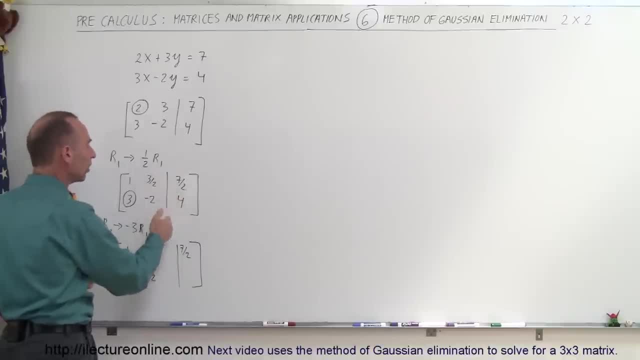 to 4,, which is a plus 8 over 2, minus 21 plus 8 is a minus 13 over 2.. Alright, you say: wow, that looks pretty mean, right. But don't worry about it, because it'll come out in. 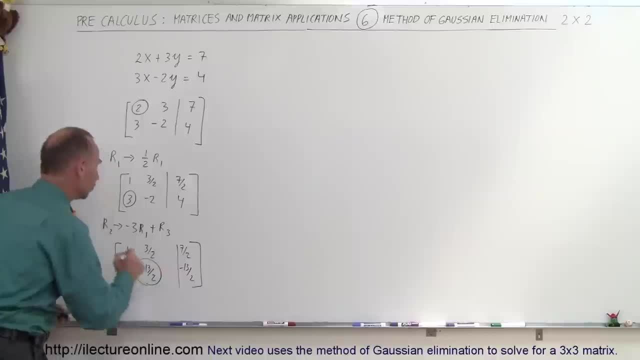 the end. The next thing we want to do is turn this into a 1.. I can do that by multiplying this row by 2 divided by 13,, or actually, negative 2 divided by 13.. So I'm going to take row. 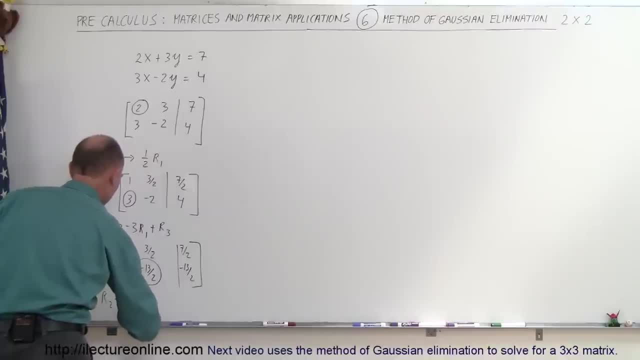 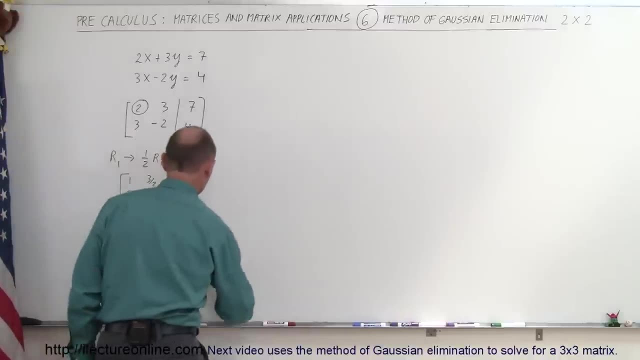 2 and replace it by negative 2 over 13 times row 2.. I turn that into a 1, and you can see I'll turn that into a 1 as well. Alright, let's go ahead and do that. So my matrix becomes: 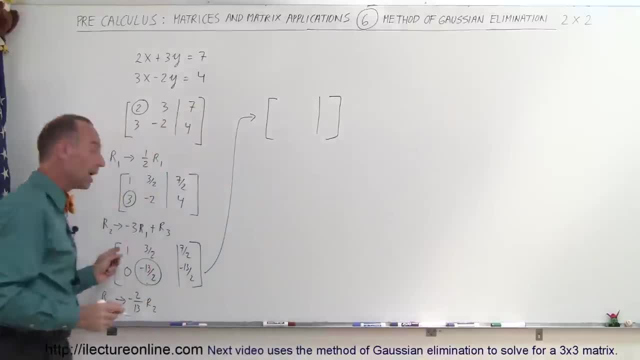 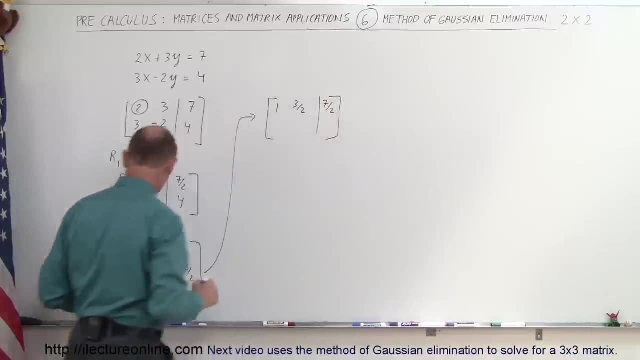 the first. So I get the following matrix. Notice that the first row will not change. I'm not meddling with the first row. so I get a 1,, a 3 halves and a 7 halves. Here I already have a 0.. Multiplying: 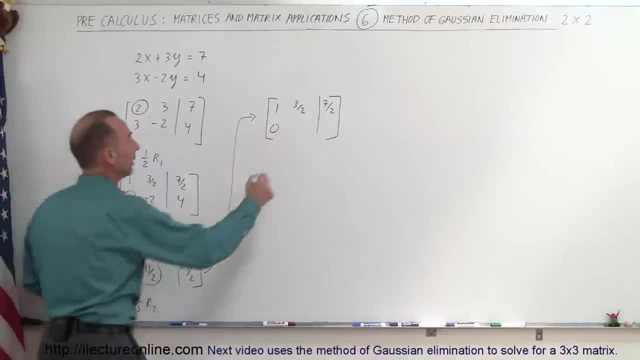 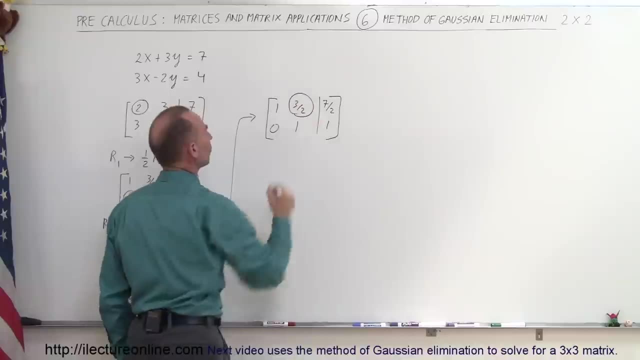 minus 13 over 2 by a minus 2 over 13 turns that into a 1, and does the same to that number over there. Alright, so now I have a 1 here. All I need to do now is get rid of this turn. 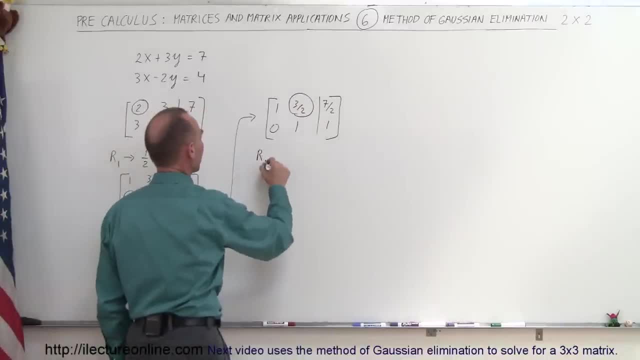 that into a 0.. I can do that by taking my first row and replacing it by the negative of that number, Times the row with the 1 in it and adding it to the original row, row 1.. If I do that, 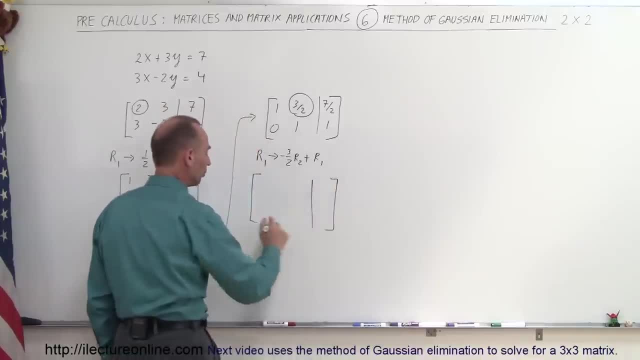 I get the following matrix: The second row does not change. I get a 0,, a 1, and a 1.. This 1 stays there Now. negative 3 halves times 1 is negative 3 halves Added to a positive. 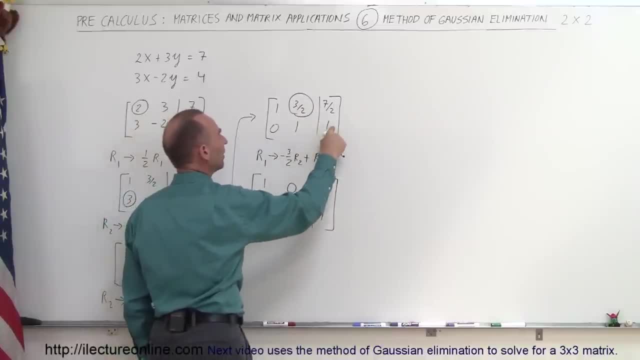 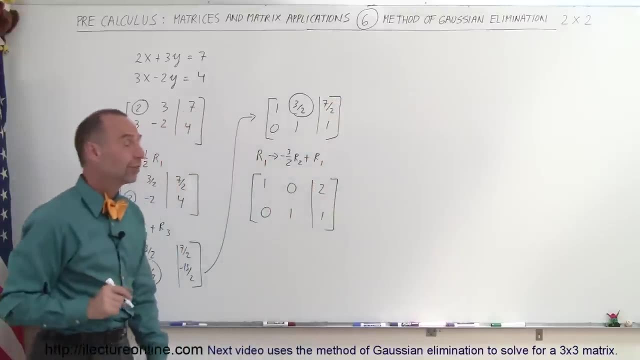 3 halves gives me 0.. Negative 3 halves times a 1 is negative 3 halves Added to a positive 7 halves gives me 4 halves, which is equal to 2.. And there's the end. I can now say that, since this row represents my x value, or I should say this column and: 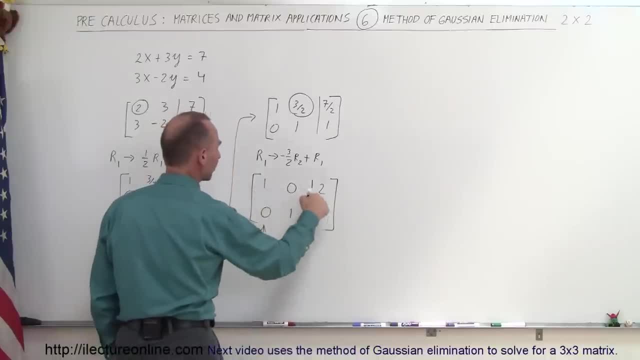 this column represents my y. I can say that 1 times x equals 2, and 1 times y equals 1, so x equals 2,, y equals 1, and that's the solution. Alright, now you may say: why go through this trouble? Why spend so much effort into solving? 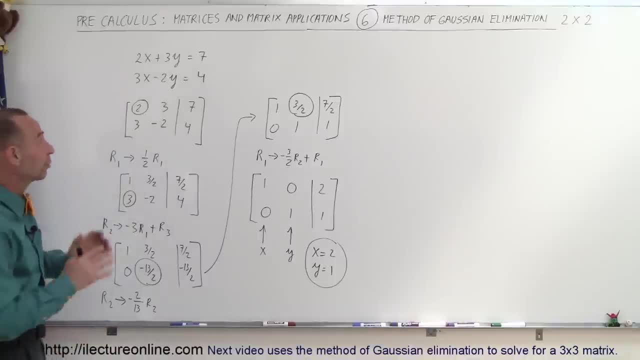 such a simple system of linear equations- And, I must admit, for a 2 by 2, for 2 equations, 2 unknowns, it's probably a little bit mundane, a little bit extra work. however, learning this technique makes it really great, because once you start doing three equations and three unknowns, and four equations and four, 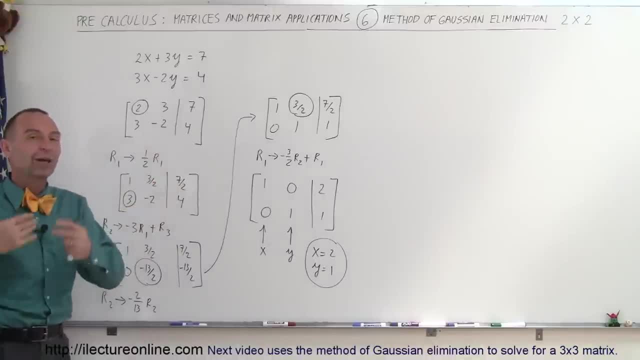 nodes. it is a lot easier to use this technique than to use the algebraic technique from before. all right, so here we know, we can see how to do a two by two equation. and now the next one: we're going to do another three by three equation. with other words, three equations and three unknowns. 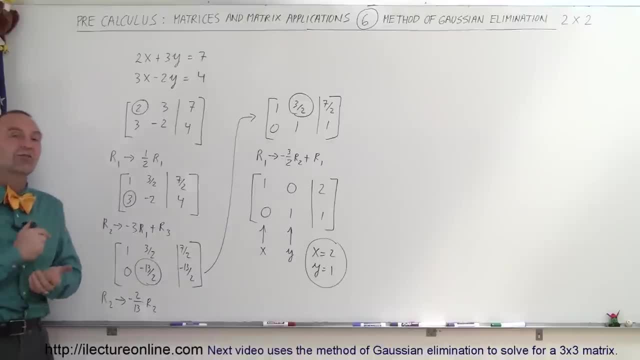 to see how to use the method of Gaussian elimination to solve systems of linear equations, and that's coming up next.